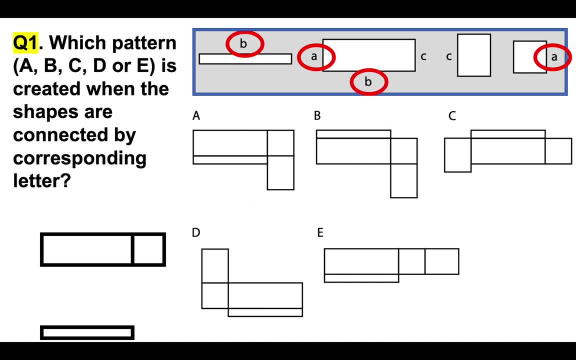 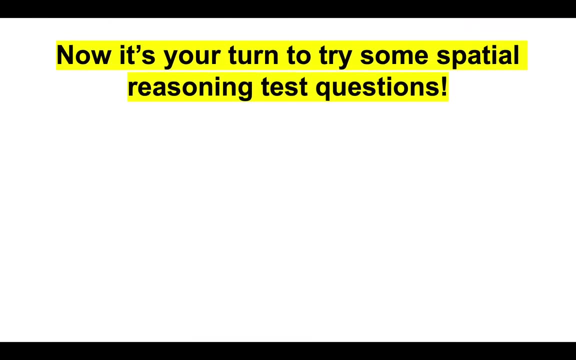 shape on the left-hand side. Then if we connect the B's together, it will come up with that shape And then finally connect the C's together to get that shape And you will notice from the answer options that the correct answer of course is C. Now it's your turn to try. 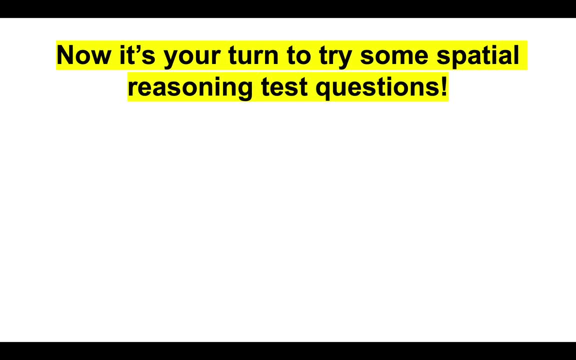 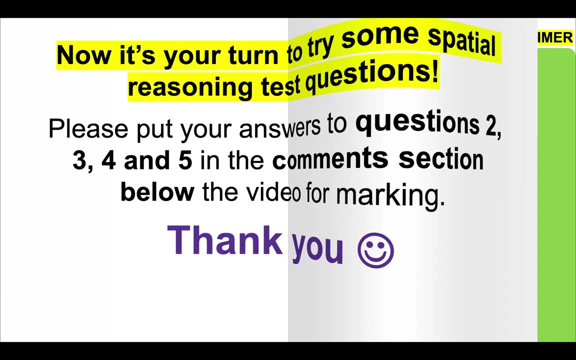 some spatial reasoning test questions that are similar to the one that I have just demonstrated. Please put your answers to questions 2, 3,, 4 and 5 in the comments section below the video for marking Thank you. I will then come on here each day and mark your answers. 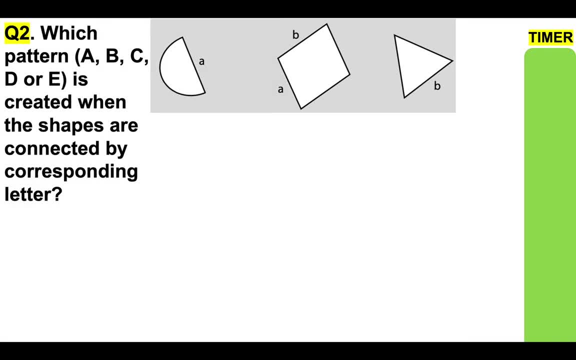 for you Now. on the right hand side of the screen, there is a green timer. You have just 10 seconds to answer each question. Question 2. Which pattern- A, B, C, D or E- is created when the shapes are connected by corresponding letter? Put your answer in the comments section. 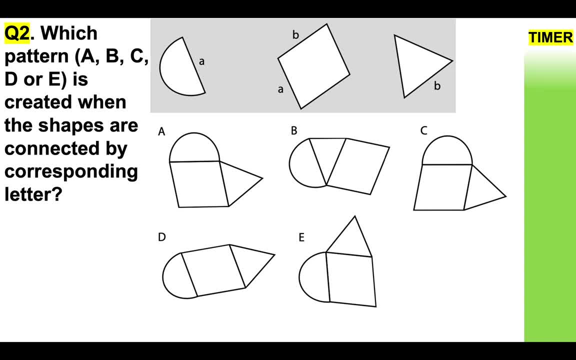 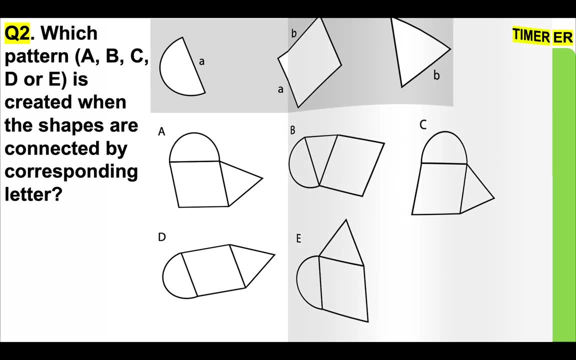 below the video. Here's a timer to question 2.. OK, well done, And of course the best way to practice any type of spatial reasoning test is to conduct lots of test practice questions. Here's question number three for you to try. 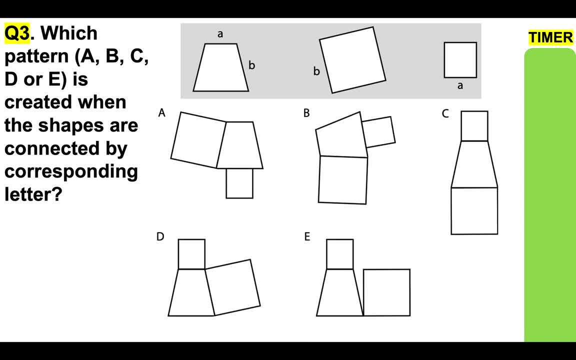 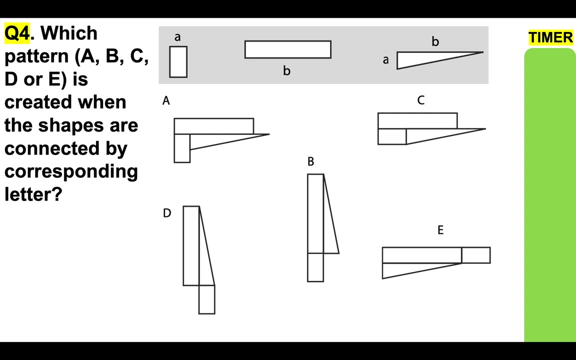 Which pattern- A, B, C, D or E- is created when the shapes are connected by corresponding letter. Here's your timer. Question number four: Again: which pattern- A, B, C, D or E- is created when the shapes are connected by corresponding letter? Here's your timer. Put your answer in the comments. 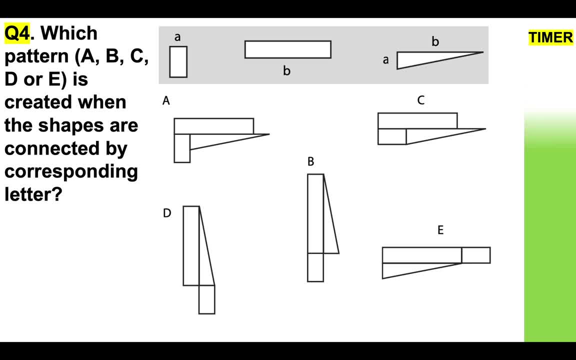 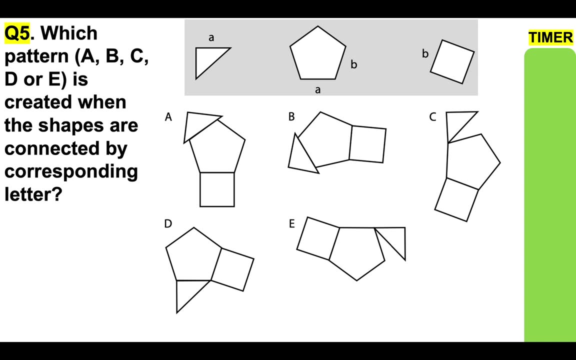 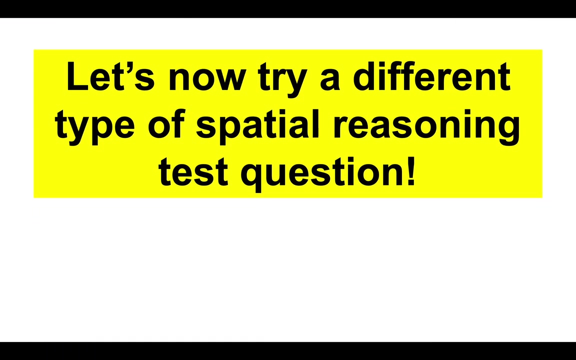 section below And the final one of this particular spatial reasoning test: Which pattern- A, B, C, D or E- is created when the shapes are connected by corresponding letter? Here's a timer. Fantastic, Well done. So let's now try a different type of spatial reasoning test question. 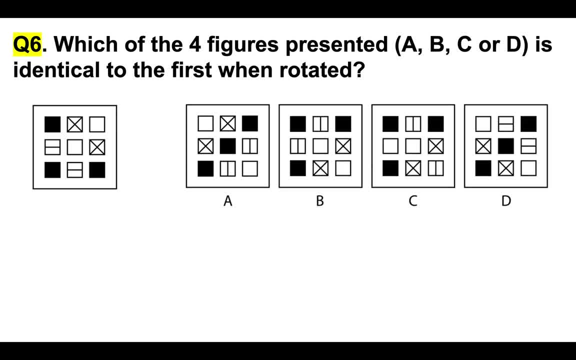 Question 6.. Which of the four figures presented- A, B, C or D- is identical to the first when rotated? So we need to look at the figure on the left And if we take one particular element of it, so we will take that bottom row of shapes- then try and find that either. 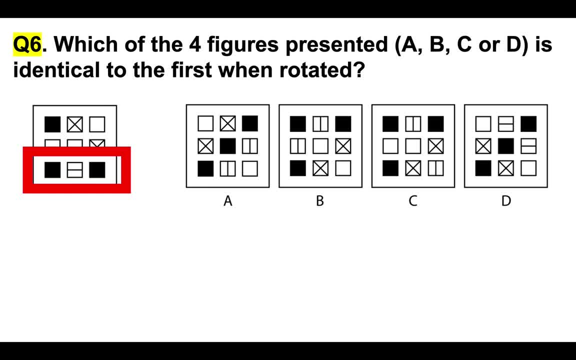 on A, B, C or D. Just use one particular area of the figure first of all, and I've chosen that part highlighted in red, and I will then work along and see whether I can see that identical when the figure is rotated within A, B, C or D. 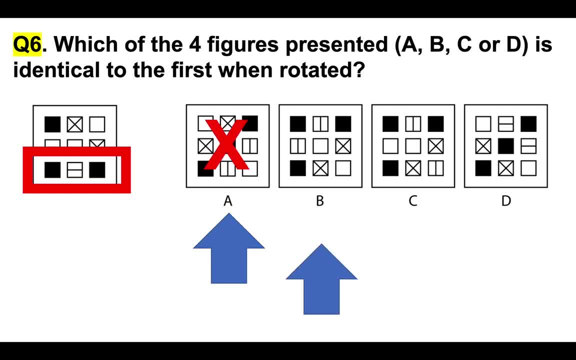 So I can't see it in A. So it's not there. I can see it in B. There it is there. When rotated, that is the same row, So it could be B. I then look at C and it is not in there. 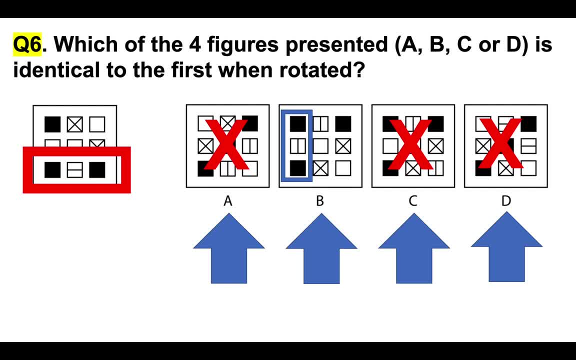 and it is not in D also. So the only answer option it can be is B, But let's just double check that. So if we then take that top row and have a look if it is configured in B and there it is, And then all we need to do is to check the middle row, There it is in. 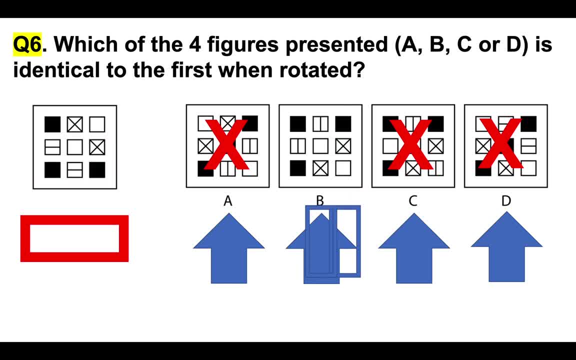 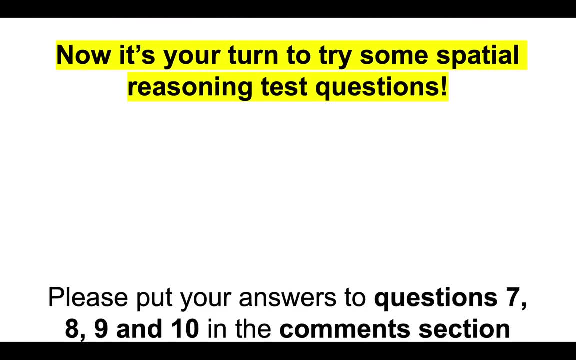 the centre. If it is configured, it's the same as the first figure, So the correct answer there is, of course, B. So now it's your turn to try some of these spatial reasoning test questions. Please put your answers to questions 7, 8, 9 and 10 in the comments section below the 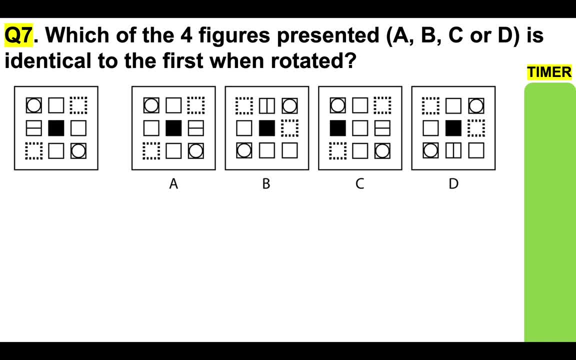 video for marking. Thank you, Same routine. We have the timer on the right hand side, Question 7.. Which of the four figures, A, B, C or D, is identical to that first one on the left when rotated? Here's a timer. 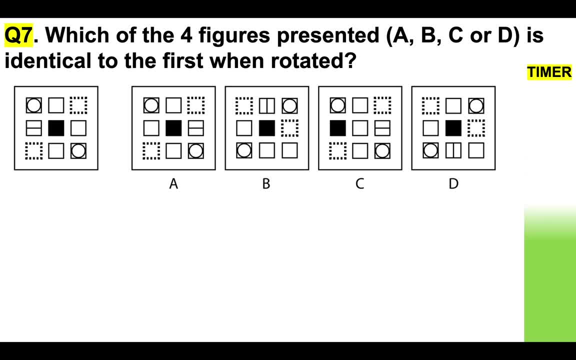 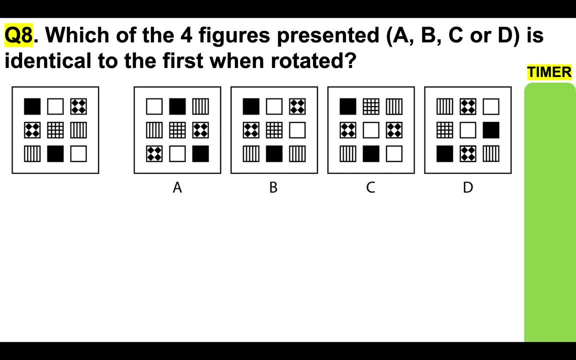 Brilliant, Well done. Question number 8.. Again, which of the four figures A, B, C or D is identical to the first on the left when rotated? Here again is your timer, And if you can get these correct within that time limit, you are doing fantastic. Thank you. 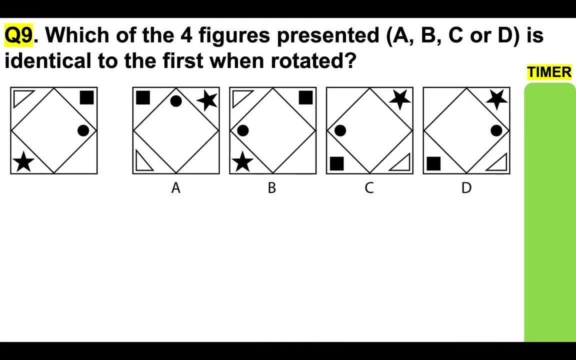 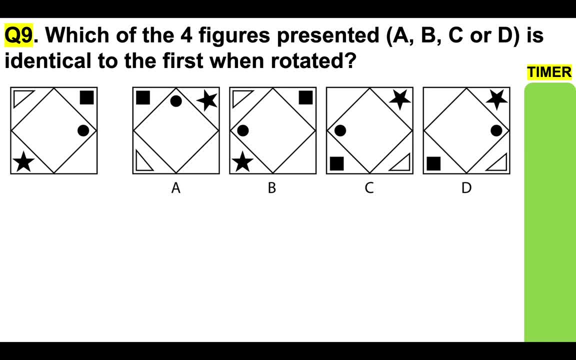 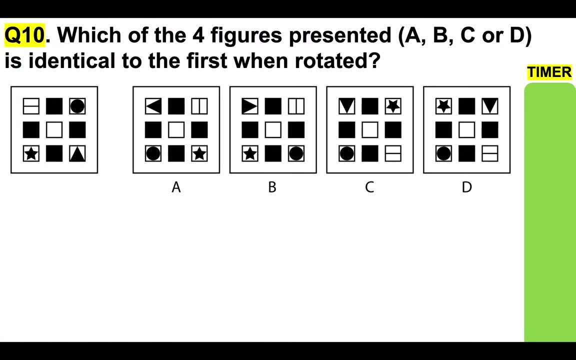 presented, A, B, C or D is identical to the first when rotated. And finally, before we move on to the next type of spatial reasoning test question, Question number 10.. Which of the four figures- A, B, C or D- is identical to the first when rotated? Put your answer. 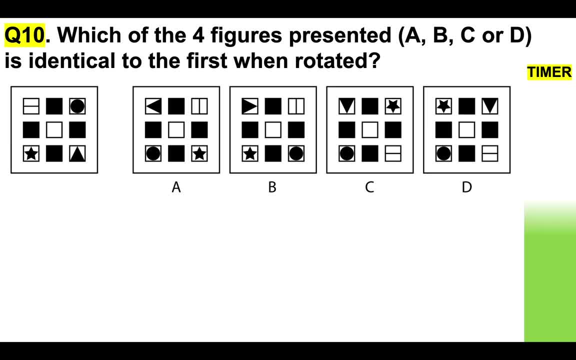 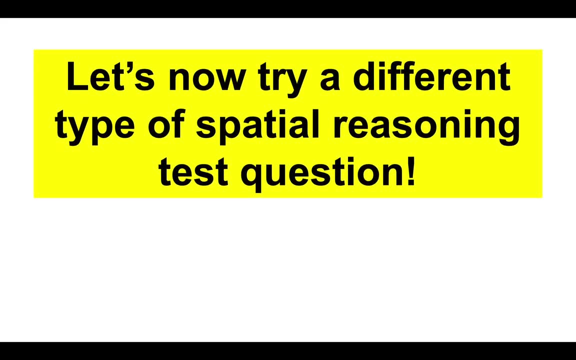 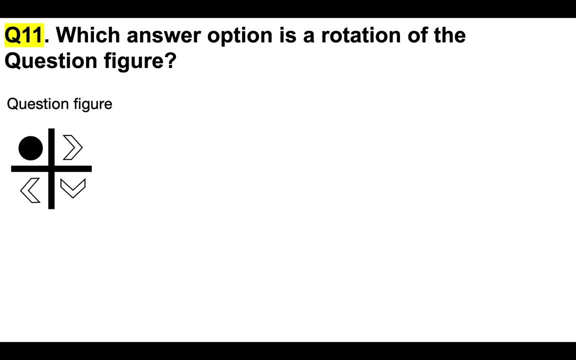 in the comments section below. Brilliant, Well done. So now let's try a different type of spatial reasoning. test question, Question 11.. Which answer option is a rotation of that question figure? Is it A, B, C, D or E? Again, instead of looking at the figure as a mass, choose one particular element of. 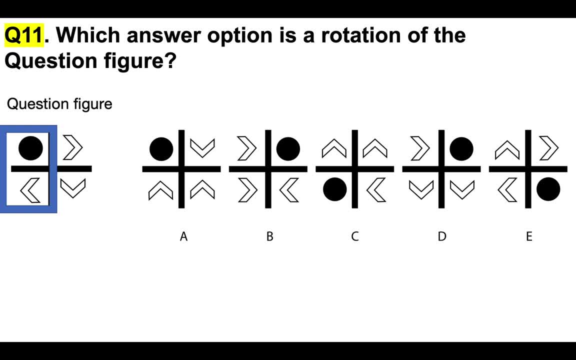 it. I'm going to choose that left column And it has that circle, the black filled in circle top left and that arrow pointing to the left at the bottom, And I will then try and find out that sequence in either A, B, C, D or E when rotated, And I can see it there on. 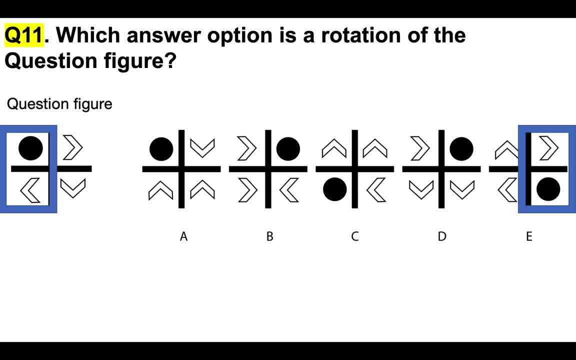 the right hand side When rotated. that's exactly what that looks like In E. I can't find it in any other. So just to confirm, I will then look at the the different arrows at the top right and the bottom right, See whether that is the same there. And it is. 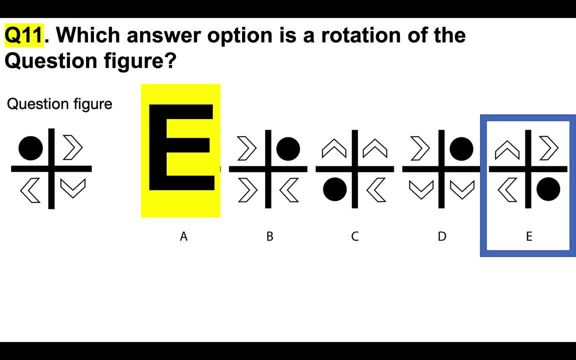 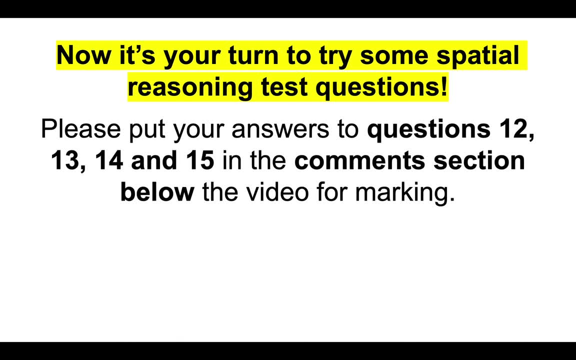 correct. So the correct answer there is E. So I'd now like you to try some of these spatial reasoning test questions Again. please put your answers to questions 12, 13,, 14 and 15 in the comments section below the video for marking. Thank you very much. So which answer? 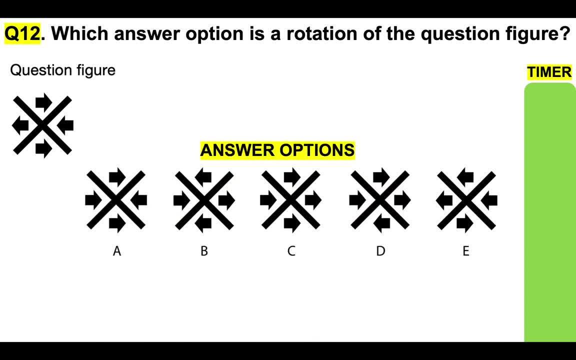 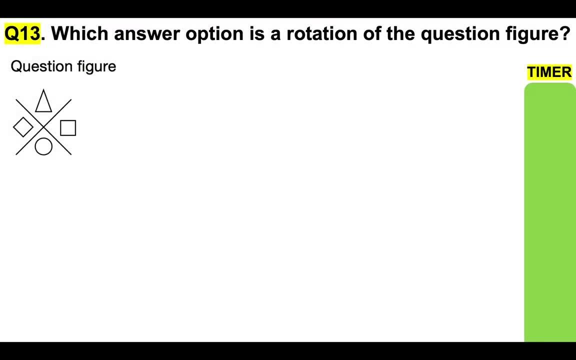 option is a rotation of the question figure. Here's your timer. Question 13.. Same again. Which answer option is a rotation of the question figure? A, B, C, D or E? Here is your timer. Put your answer in the comments section below, please.